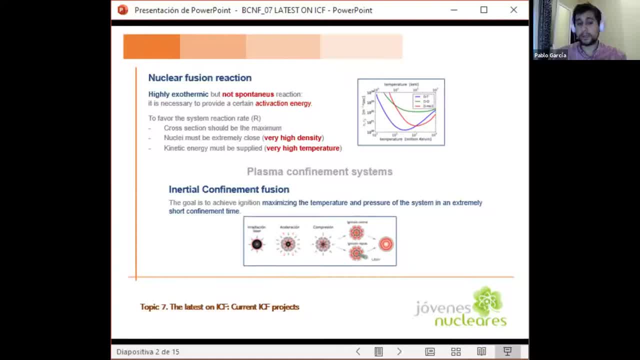 We will favor the reaction by raising two parameters, temperature and pressure, up to an extremely high point Where we will get a plasma. And, as you have already been told, one of the ways to control and manipulate plasma is the inertial confinement, or IC fusion. 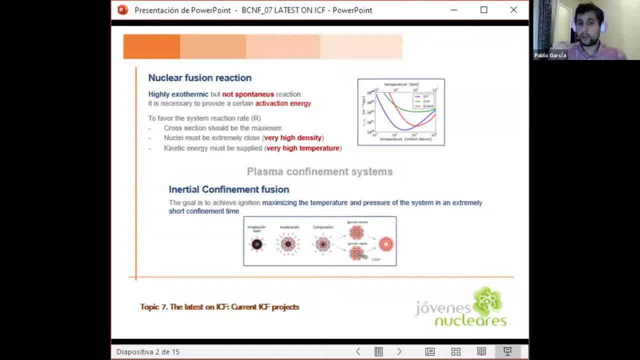 Where we look for ignition to happen in an extremely short confinement time, maximizing both the temperature and the pressure of the system. IC is based on shooting these small plastic capsules filled with deuterium and tritium. These capsules are placed into a great vacuum chamber and heating them very much with really high power pulsed lasers. 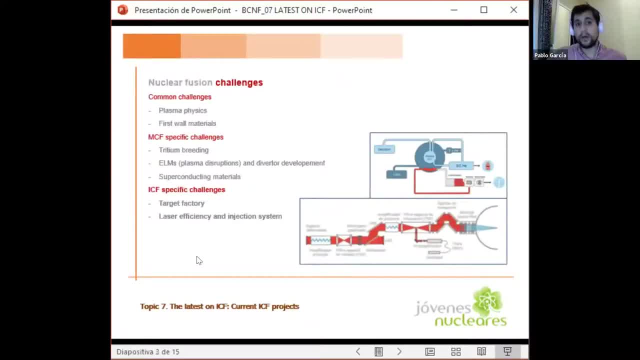 And just to end with a brief resume of the road so far. you already may know that we are still facing major challenges to reach a commercial operating fusion reactor And that the schedule depends on fusion related laboratories to solve all these challenges. you can see in the slide. 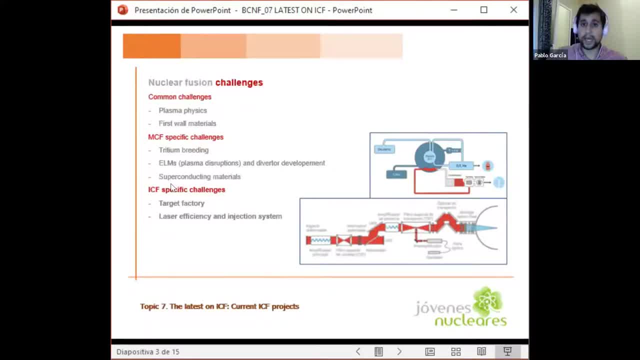 Common challenges: magnetic confinement challenges, IC challenges. So we've just reviewed the main facility that is trying to overcome magnetic confinement challenges- this ITER project- And now we are doing the same for the inertial confinement. So where is nuclear fusion today? 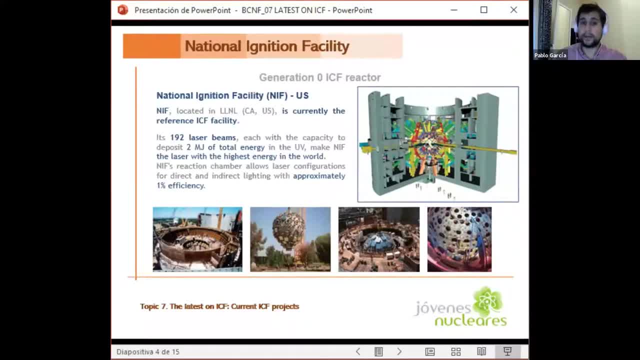 You just saw ITER. And if we compare nuclear fusion with the development of nuclear fission reactors, if I have to be completely sincere- and I know this will disappoint many of you- we are still in generation zero reactors, just like the first Chicago Pile 1 fission reactor, which was a pure research facility back in the 1940s. 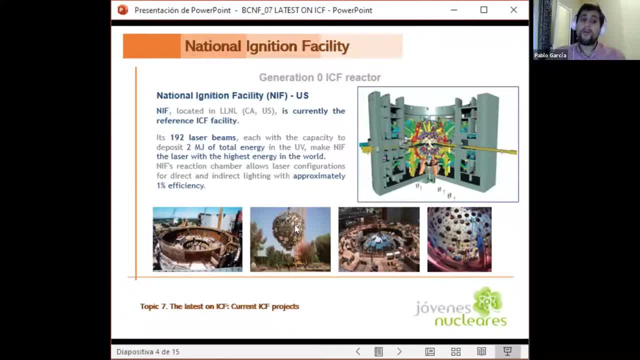 And the main one of those research facilities- and naturally big laboratories- dedicated to IC fusion, to inertial confinement fusion research, is the National Ignition Facility located in California in the United States, And it's currently the reference ICF facility. It's 192 laser beams. it's with the capacity to deposit 2 megajoules of total energy. 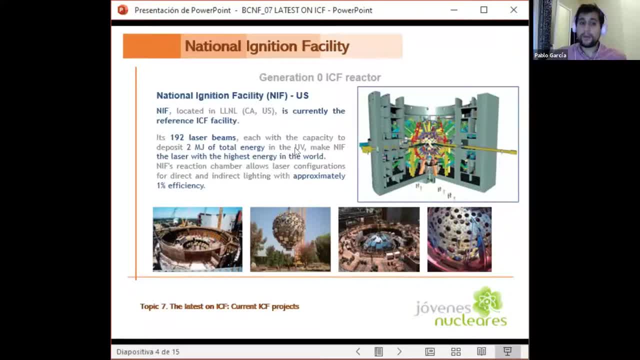 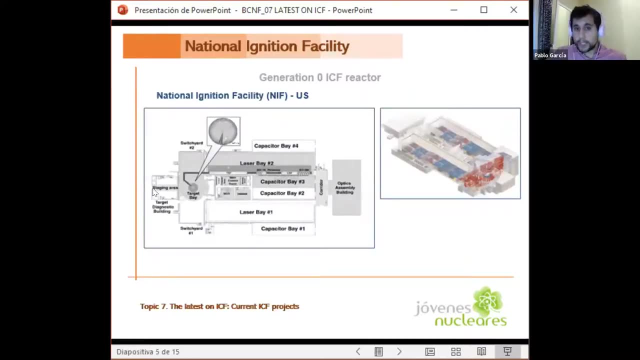 make NIF a laser with the highest energy in the world. NIF's reaction chamber allows laser configuration both for direct and indirect lightning of the target with approximately 1% efficiency. In these images you can see what NIF is like. 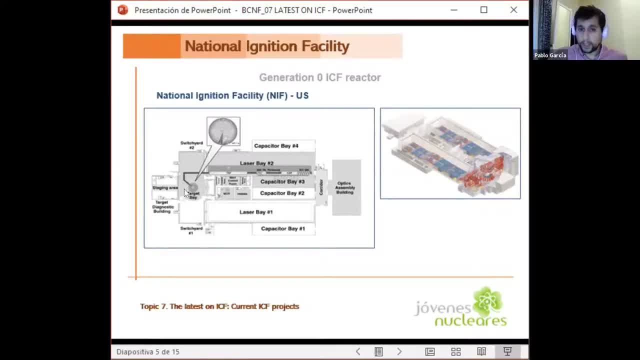 And it's just remarkable that the vacuum chamber here, where the magic comes through, it's only a small part of the facility, which mainly consists on allocating- you can see- all these spaces to allocate all the laser beams, related equipment And, as I told at the beginning of the presentation, 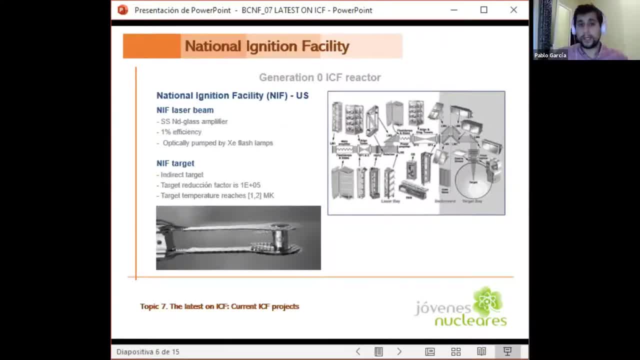 for my lecture. I'm not going to explain any technical details about NIF, but I think it's important to remark that, as the reference IC facility, NIF- the National Ignition Facility- lightning is on an indirect target, as you can see in this figure. 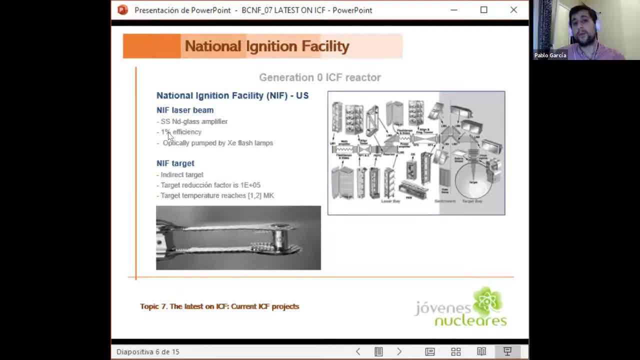 and that we are working with laser efficiency up to 1%. So this means that if we want to deposit 2 megajoules- 2 megajoules of energy- in the target, we need to generate a 200 megajoule laser in the very first moment. 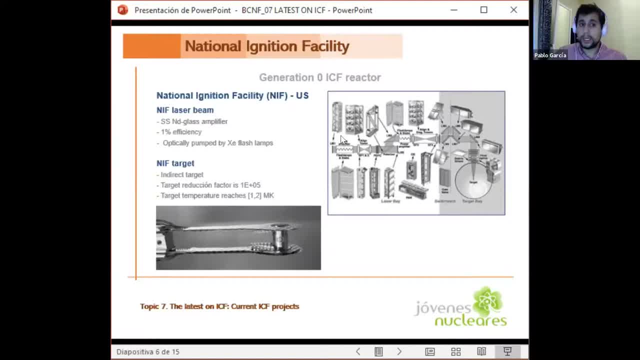 because part of that energy gets lost in each and every optical event on this component, as you can see in this laser system description figure, And that is the reason why we say that laser efficiency is one of the major challenges on inertial confinement fusion. 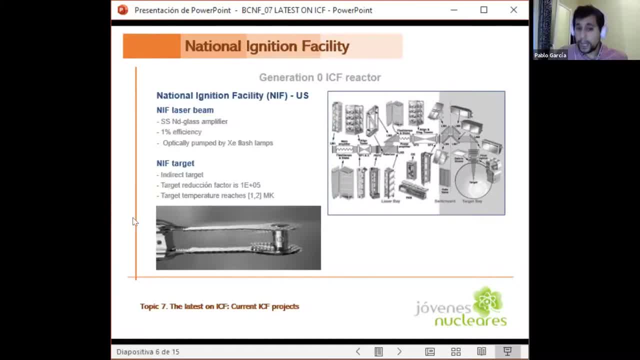 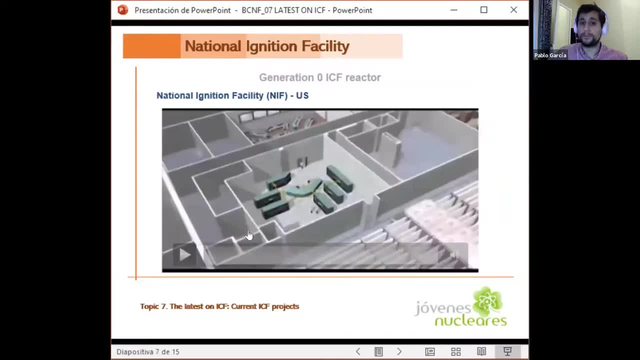 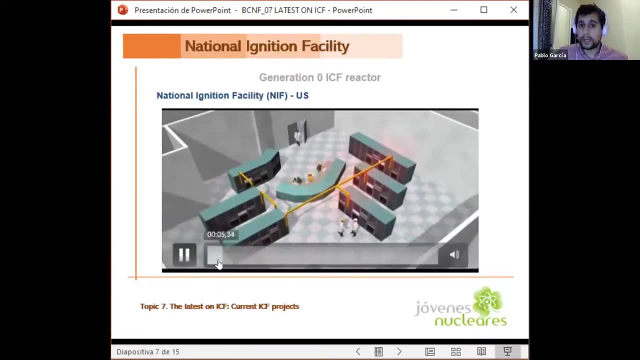 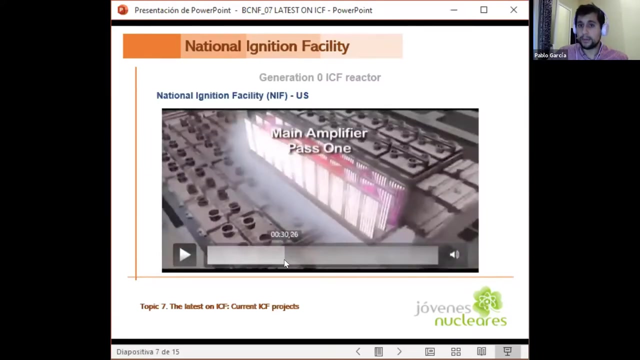 If we don't improve this topic, it would be absolutely impossible to get a profitable inertial fusion reactor. Well, here you can see a brief video that shows how NIF works and how the laser beams are generated and are amplified several times. The beams are also collimated. 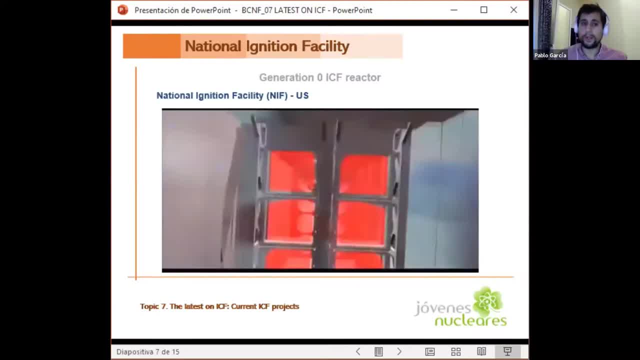 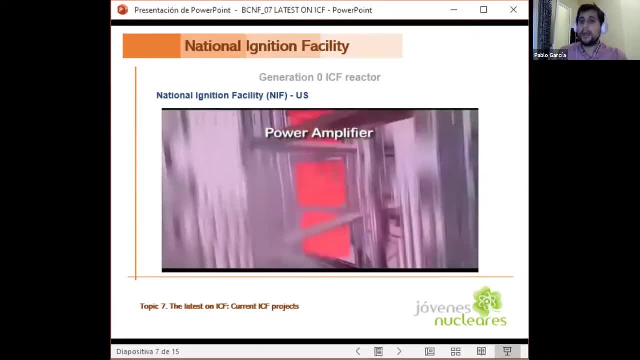 which means something like a tint or in terms of light. we try to that every photon in the beam has the same energy, And then they are. as I mentioned, they are amplified several times, Then they are focused next to the vacuum chamber. 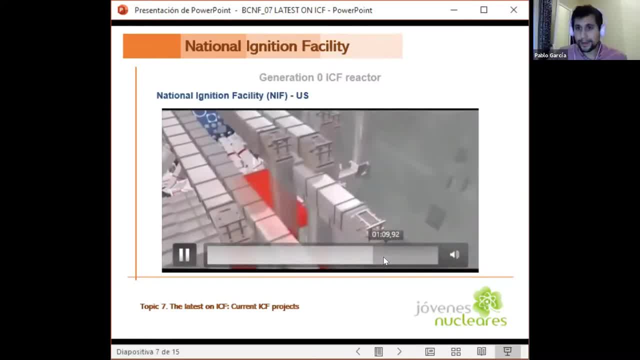 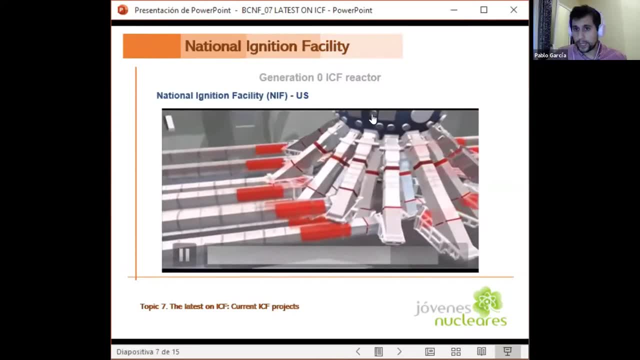 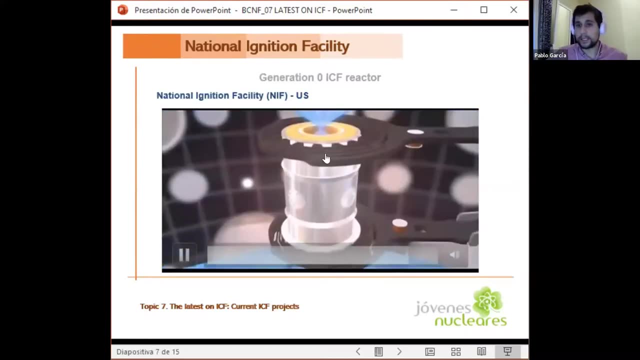 They are up here, rising, reaching the vacuum chamber. So here they are, focused on the vacuum chamber And they are shot to light the target And, as we just said, this lightning is an indirect lightning. Finally, as this is inertial confinement. 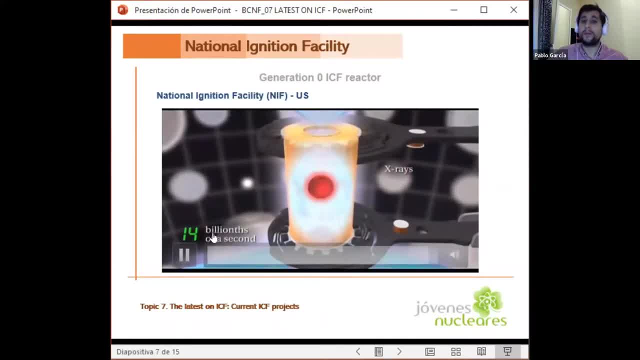 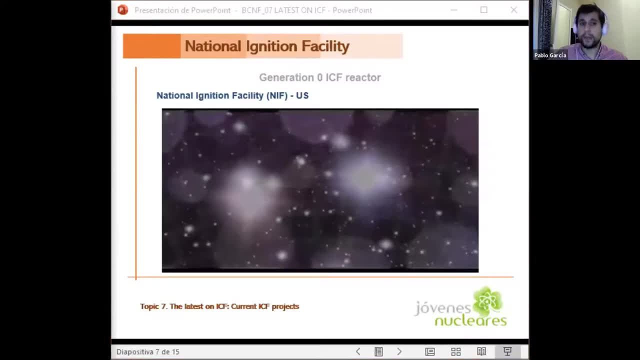 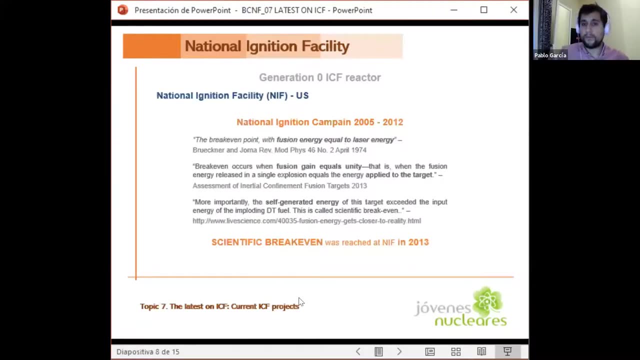 we get the ignition in an extremely short confinement time. Here you can see 20 billions of seconds. This is the confinement time. So I know I have mentioned too many times the challenges of IC and I don't want you to leave this course. 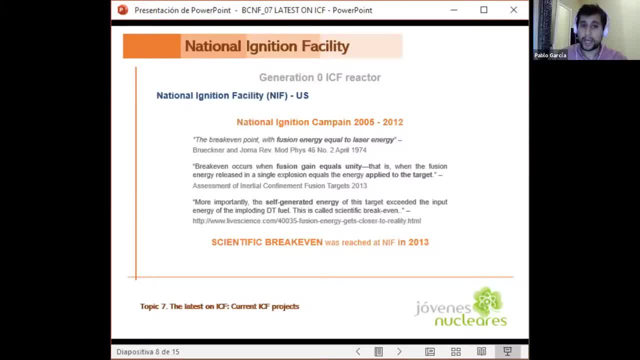 So I have to remark that in 2013,, NIF reached the so-called break-even event, which means that we got, for the first time, more energy from the fusion reaction than what we put on the target. This does not include the energy we spent in generation. 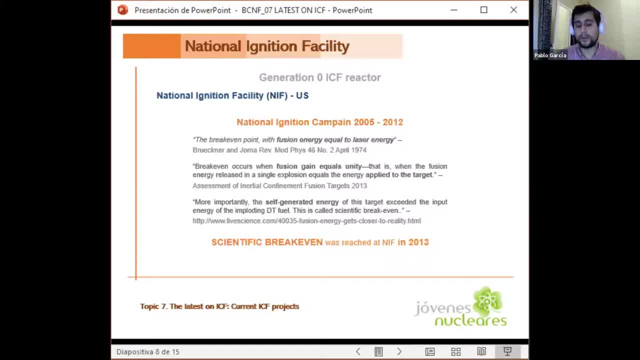 in generating the laser beams and gets lost due to the low laser efficiency. But it's still really good news. And well, we said that NIF, the National Ignition Facility, is currently the reference inertial confinement fusion facility, but it's not the only one. 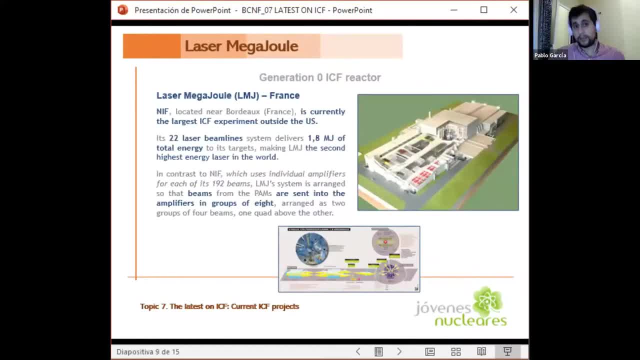 We can talk also about the laser megajoule located in France, which is the largest ICF experiment outside the United States. LMJ has 22 laser beam lines. Each of them delivers 1.8 megajoules of total energy to the target. 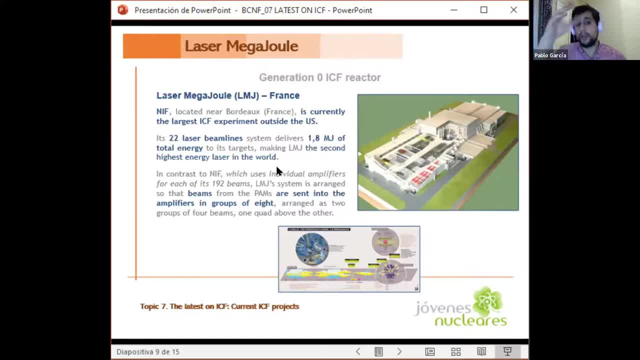 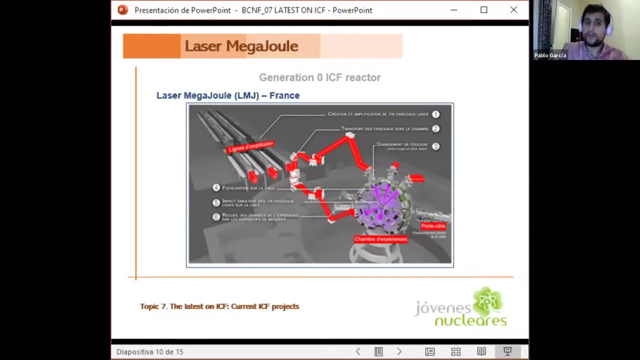 And it does it in indirect lightning- Just a little lower than NIF, Which is the most significant difference between LMJ and NIF. Well, in contrast to NIF, which uses individual amplifiers for each of its 192 beams, LMJ's system is arranged. 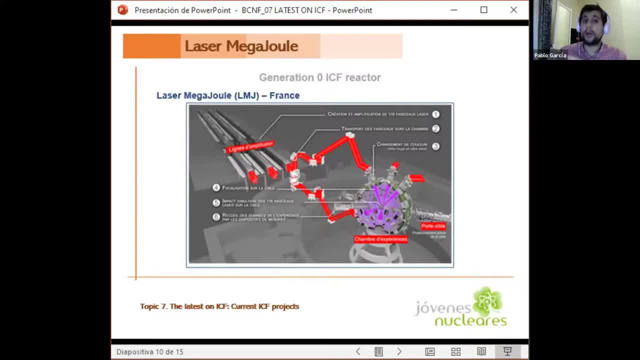 so that beams are sent into amplifiers in groups of eight, arranged as two groups of four beams, one quad above the other. So this is really a really big advance in terms of laser efficiency. We are not needing 200 lasers, but just about 20 lasers. 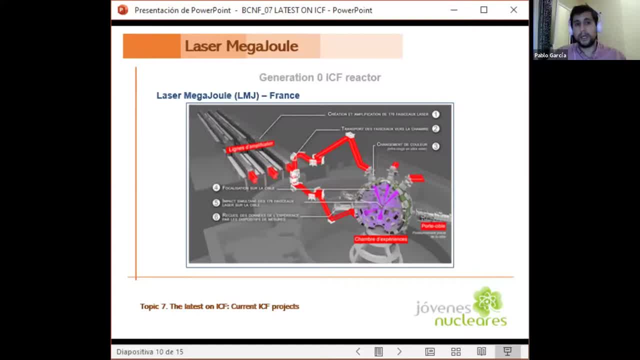 to get almost the same energy. So it's a really big advance in laser efficiency. Well, finally, as you just saw, for magnetic confinement, we have to work with this NIF and LMJ facilities until we fully have understood plasma And develop the materials. 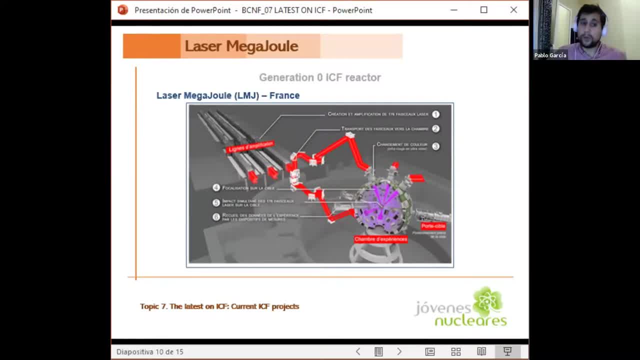 and associated technologies. we will need to operate an energy-profitable reactor, And then we will have to prove that this kind of reactors are economically profitable too. We will need to build demonstration IC power plants, And one of these projects Generation 1 ICF reactors. 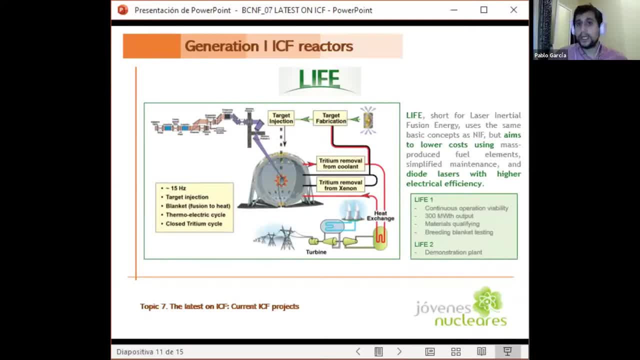 or inertial confinement demonstrators, is LIFE. LIFE, as you can see in the screen, is an evolved version of NIF that aims to lower costs. Actually, it is planned to use a national emission facility and adapt it to become LIFE. But I have to say 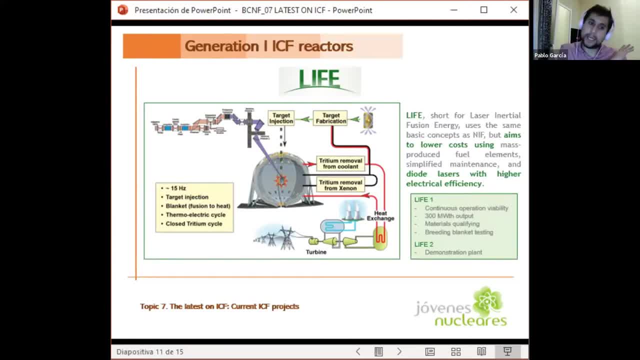 that this project is now frozen because, although I said that NIF reached the break-even in 2013,, well, this experiment has not achieved its ignition-related goals yet, So it's not a total success And it has impacted in LIFE's schedule. 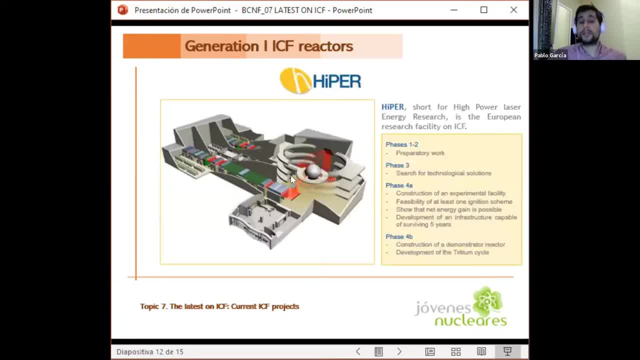 The other project which is under consideration is HYPR, which is the European proposal, And in this case you can see we are still really far from Phase 4b, But it's remarkable that HYPR is planned to be designed with a fast-ignition approach. 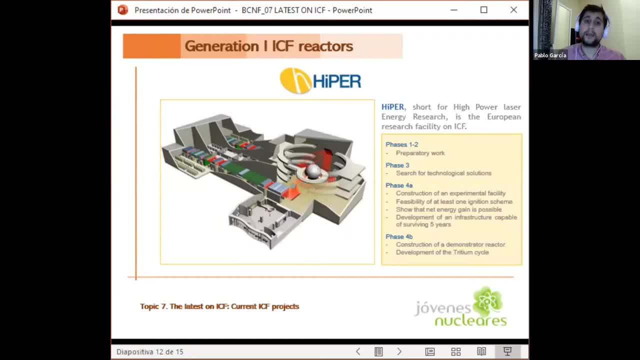 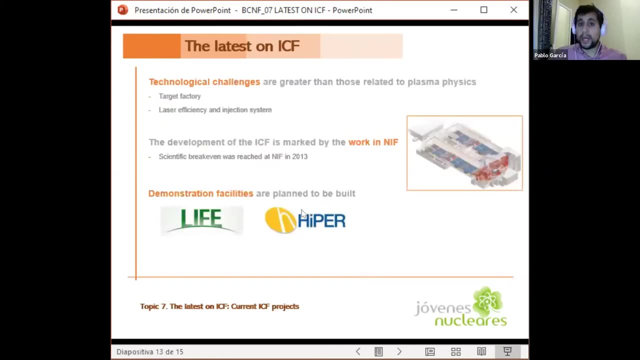 which uses much smaller lasers than conventional ICF facilities or designs but yet produces fusion power outputs about the same magnitude. So it's a really interesting approach to ICF, And I hope I fit it to time. so just three sentences to resume this lecture.